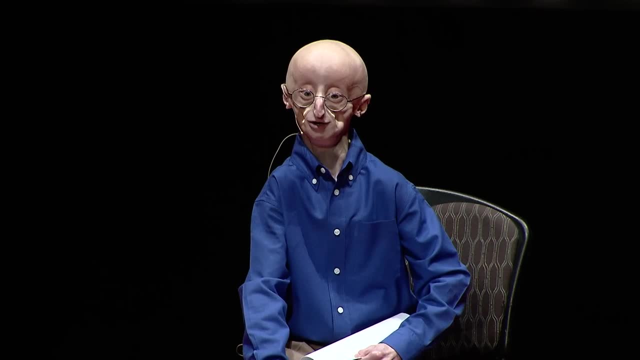 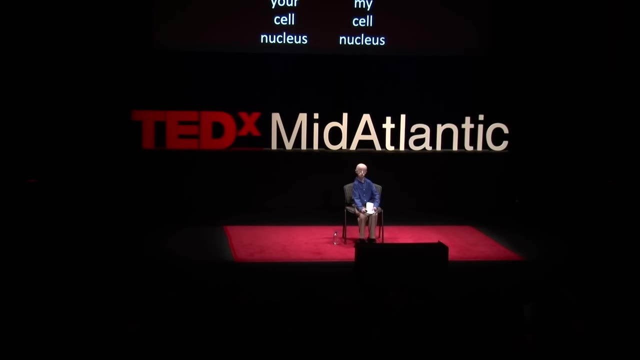 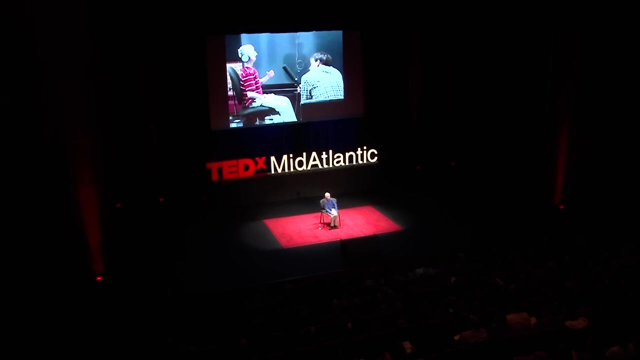 lack of weight gain, stinted growth and heart disease. Last year, my mom and her team of scientists published the first successful progeria treatment study and because of this I was interviewed on NPR and John Hamilton asked me the question: what is the most important thing? 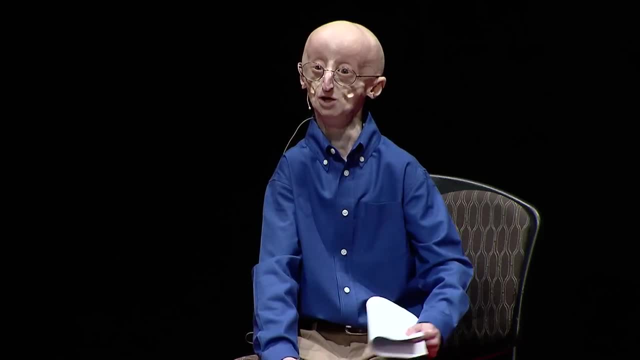 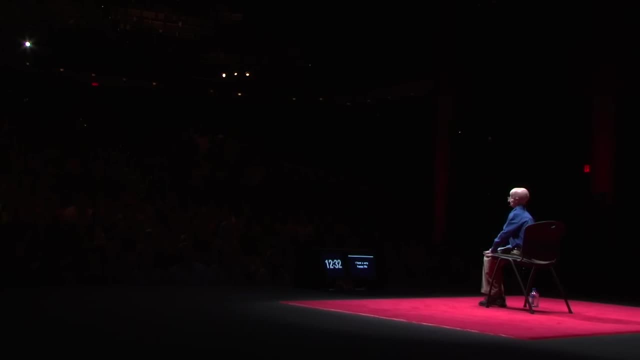 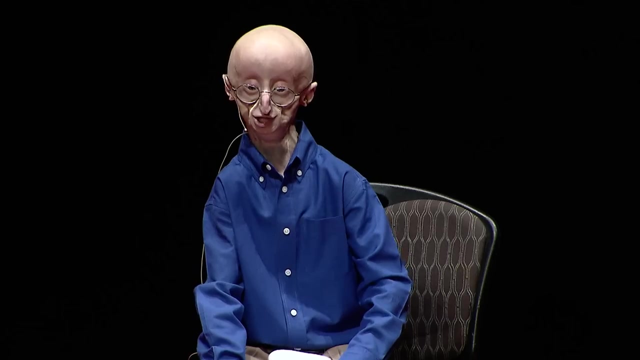 that people should know about you, And my answer was simply that I have a very happy life. So, even though there are many obstacles in my life, with a lot of them being created by progeria, I don't want people to feel bad for me. I don't think about these obstacles all the time. 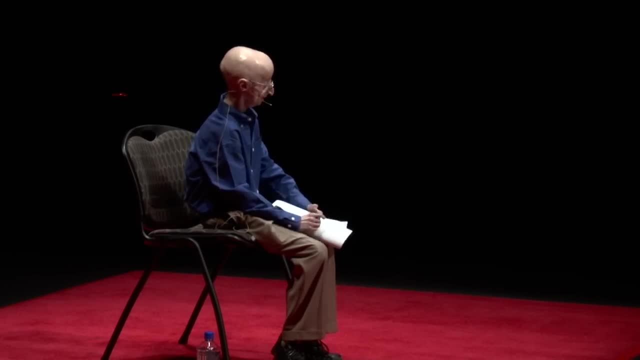 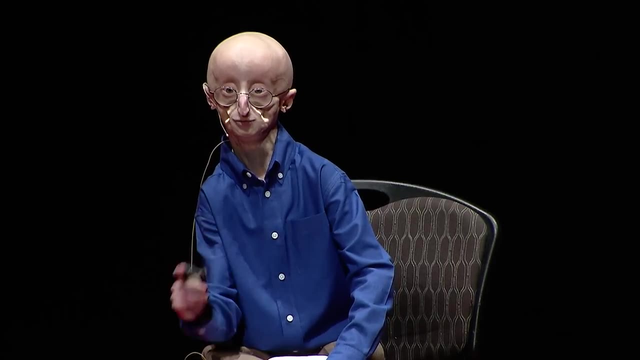 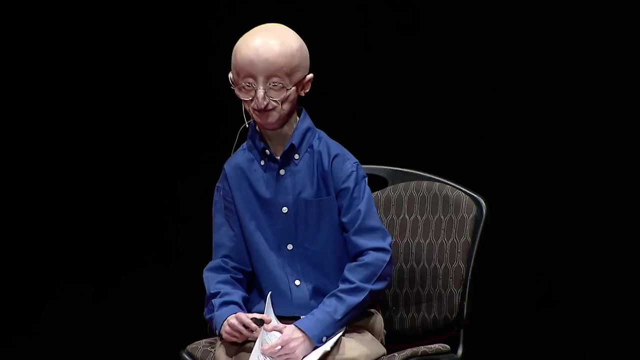 and I'm able to overcome most of them anyway. So I'm here today to share with you my philosophy for a happy life. So for me, there are three aspects to this philosophy. So this is a quote from the famous Ferris Bueller. The first aspect to my philosophy is that I'm okay with what I 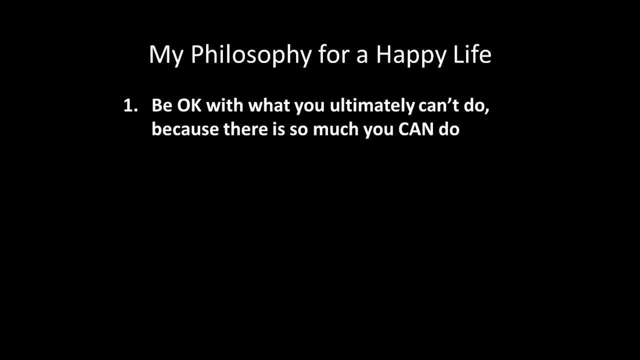 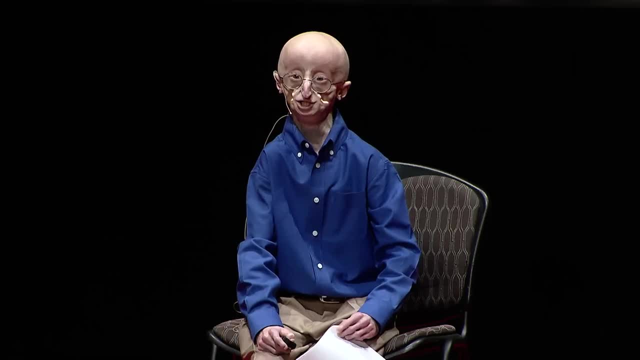 ultimately can't do because there's so much that I can do. Now people sometimes ask me questions like isn't it hard living with progeria, Or what daily challenges or progeria do you face? And I'd like to say that I'm okay with what I ultimately can't do because there's so much that I can do. 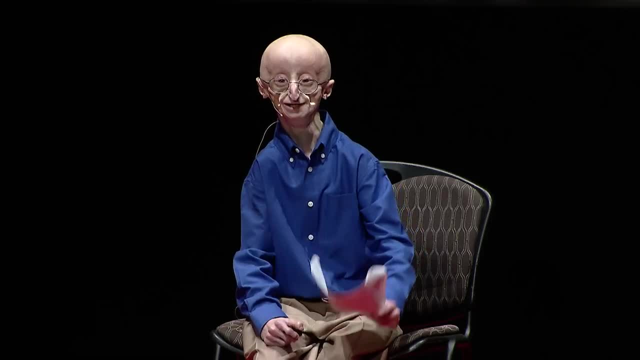 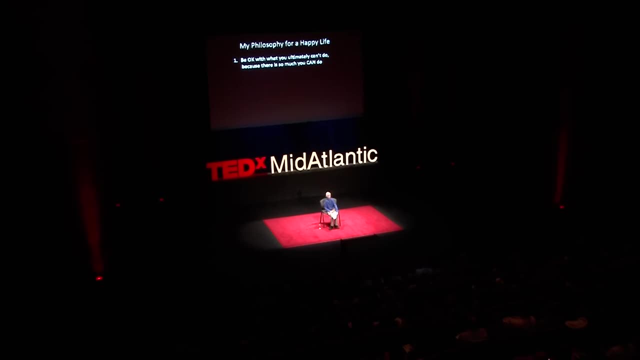 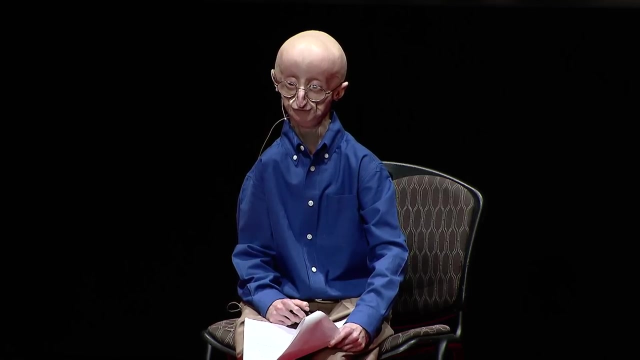 So, even though I have progeria, most of my time is spent thinking about things that have nothing to do with progeria at all. Now, this doesn't mean that I ignore the negative aspects of these obstacles. When I can't do something like run a long distance or go on an intense roller coaster. 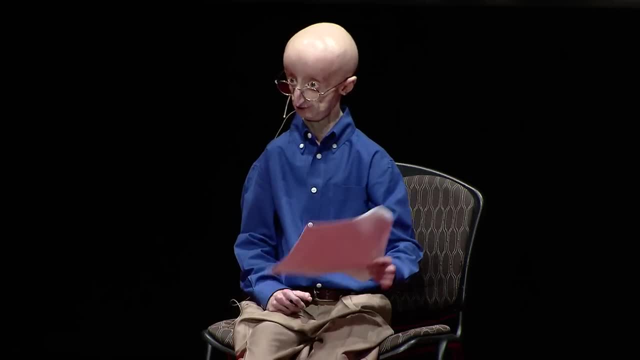 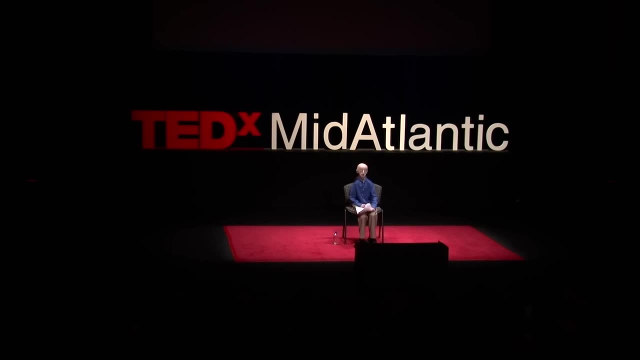 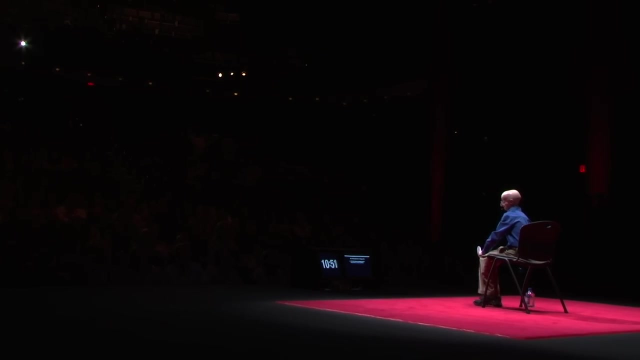 you know, I know what I'm missing out on, But instead I choose to focus on the activities that I can do through things that I'm passionate about, like scouting, music or comic books or any of my favorite Boston sports teams, Yeah. So, however, 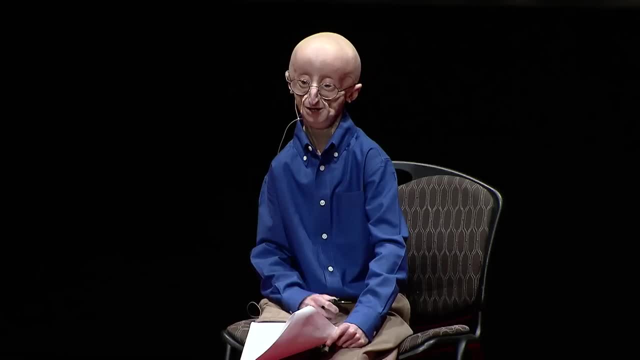 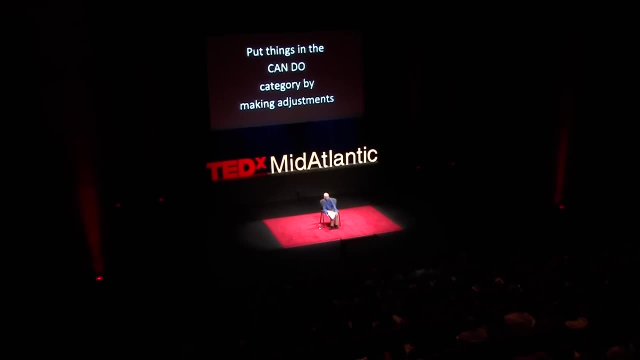 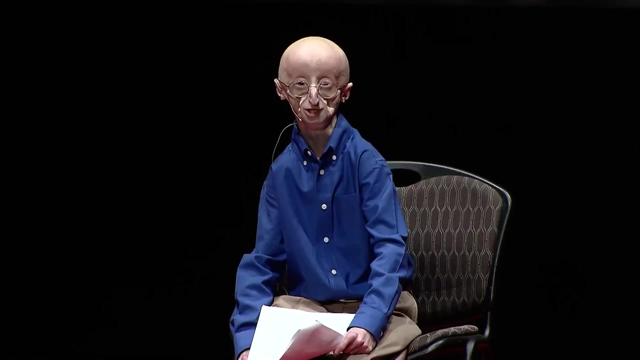 sometimes I need to find a different way to do something by making adjustments, And I want to put those things in the can-do category, kind of like you saw with the drum earlier. So here's a clip with me playing Spider-Man with the Foxboro High School marching band at halftime. a couple 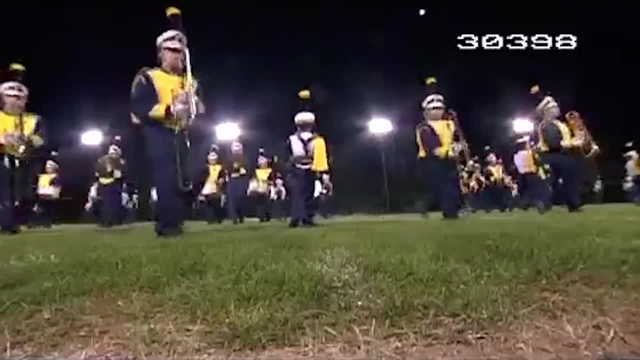 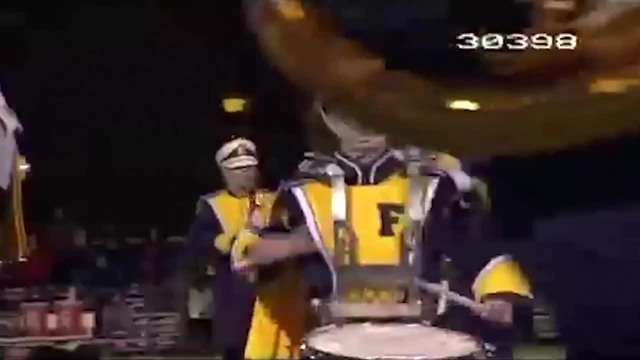 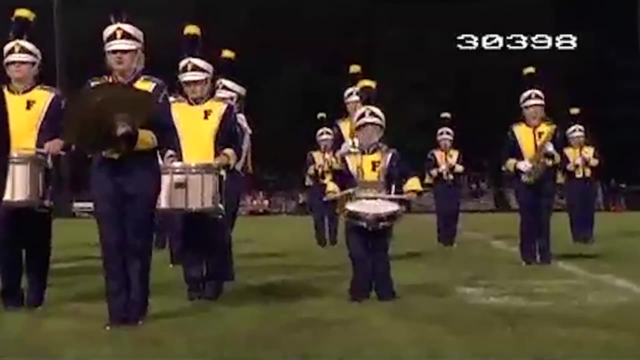 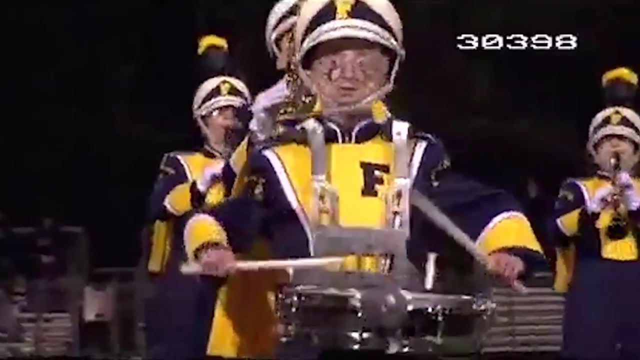 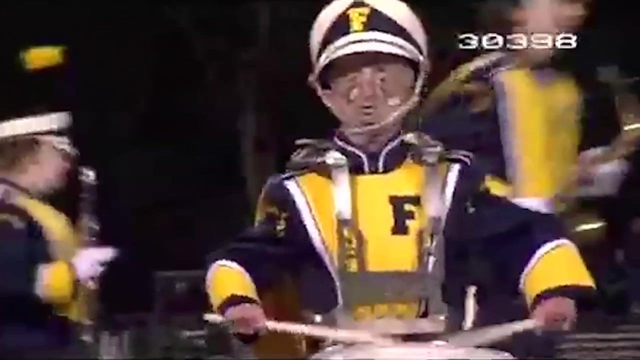 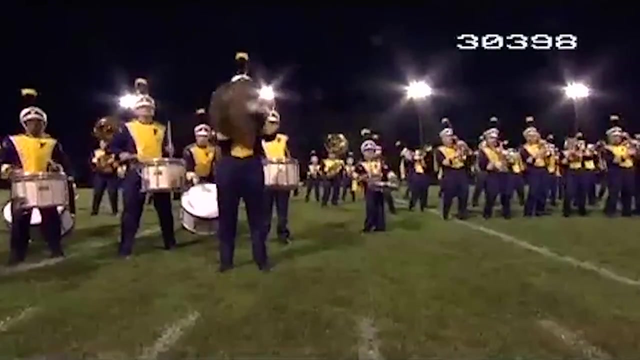 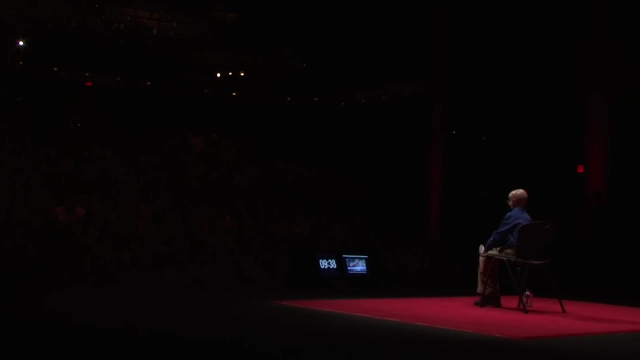 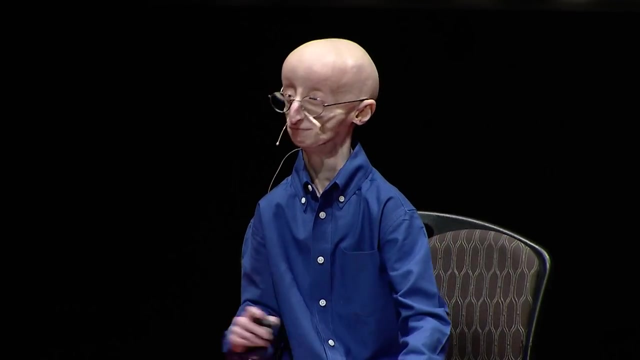 years ago. So here's a clip with me playing Spider-Man with the Foxboro High School marching band. So here's a clip with me playing Spider-Man with the Foxboro High School marching band. Thank you, All right. all right. So that was pretty cool, And so I was able to accomplish my dream. 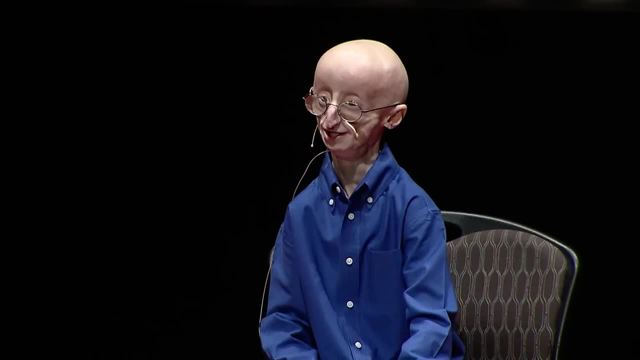 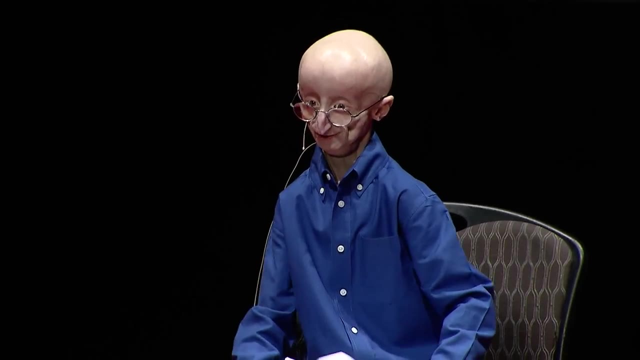 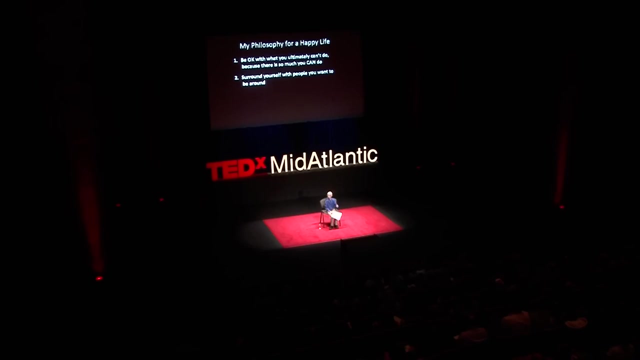 of playing snare drum with the marching band, as I believe I can do for all of my children. So hopefully you can accomplish your dreams as well with this outlook. The next aspect to my philosophy is that I surround myself with people that I want to be with. 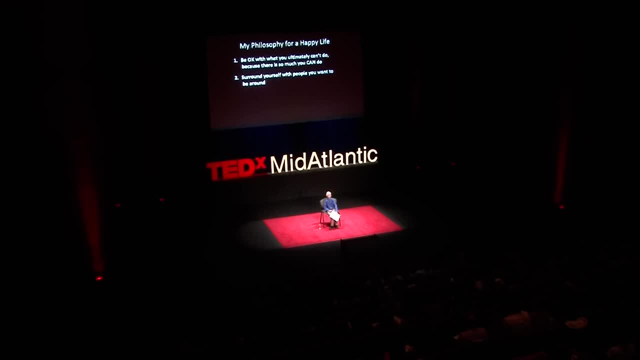 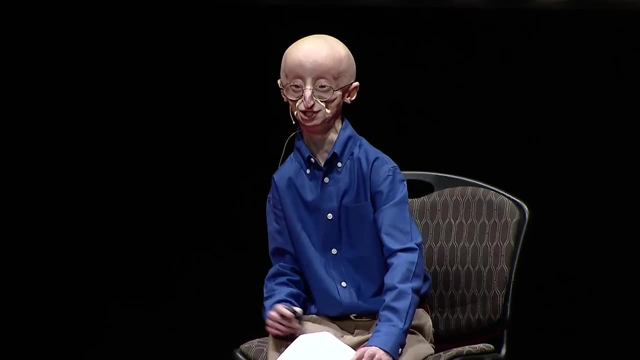 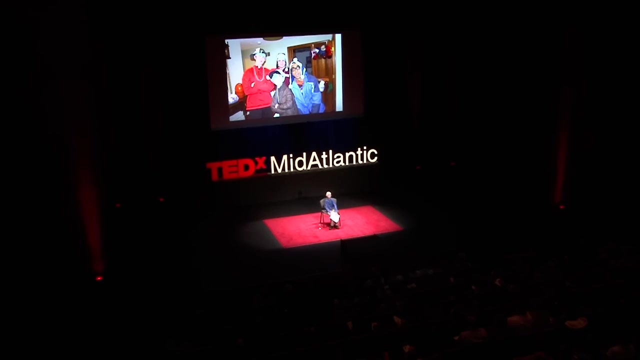 people of high quality. I'm extremely lucky to have an amazing family who have always supported me throughout my entire life, And I'm also really fortunate to have a really close group of friends at school. Now we're kind of goofy- A lot of us are band geeks- but we really enjoy each other's company. 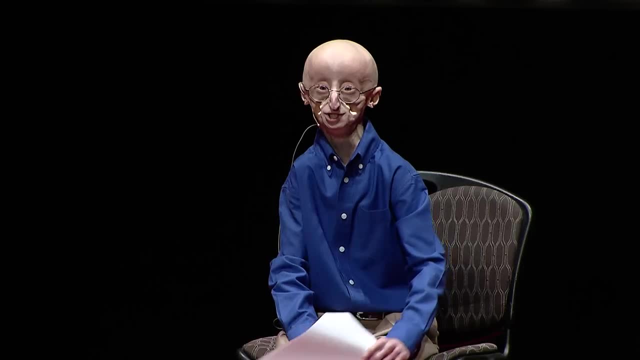 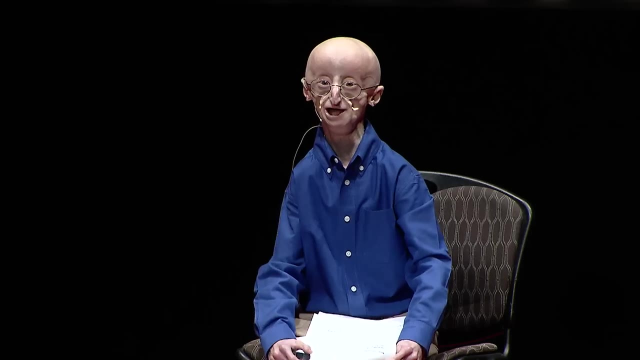 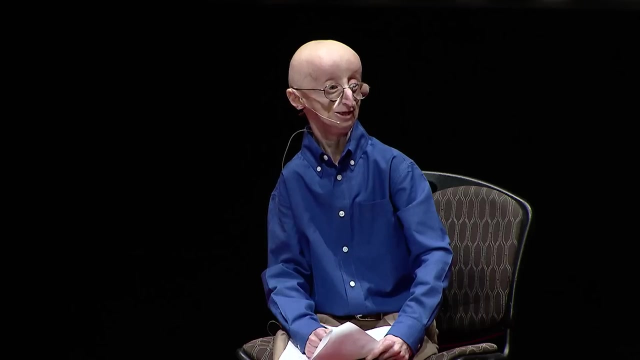 and we help each other out when we need to. We see each other for who we are on the inside. So this is us goofing off a little bit, And so we're juniors in high school now and we can now mentor younger band members as a single collective unit. 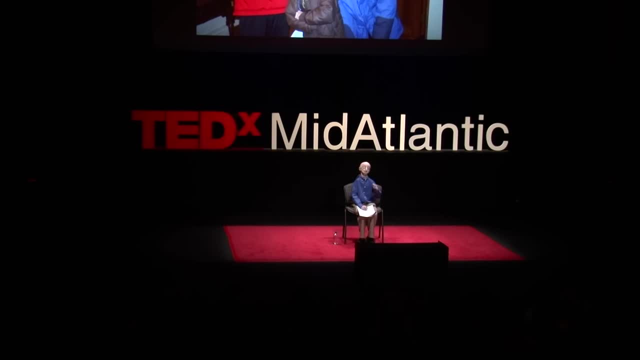 What I love about being in a group like the band is that the music that we make together is true, it's genuine and it supersedes progeria, So I don't have to worry about that when I'm feeling so good about making music. 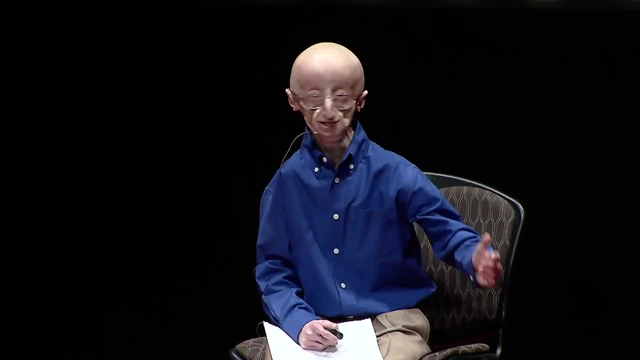 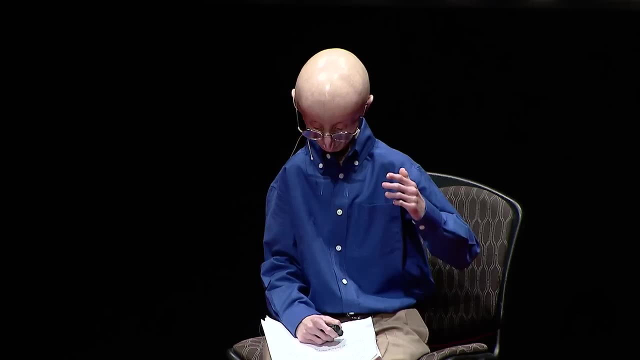 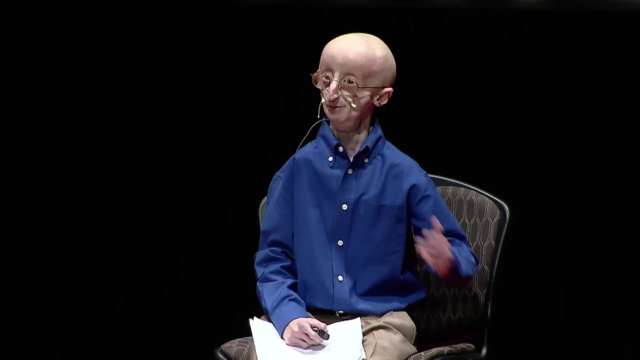 But even having made a documentary and going on TV a couple times, I feel like I'm at my highest point when I'm with the people that surround me every day. They provide the real positive influences in my life, as I hope that I can provide a positive influence in theirs as well. 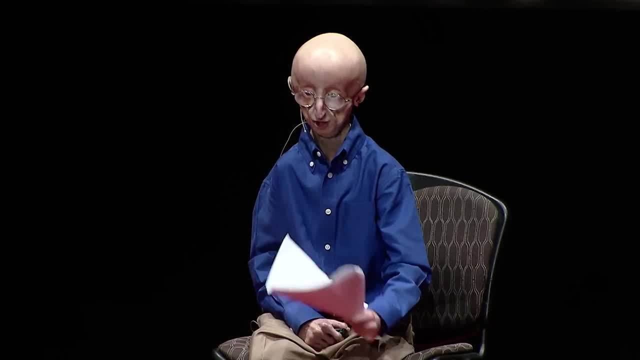 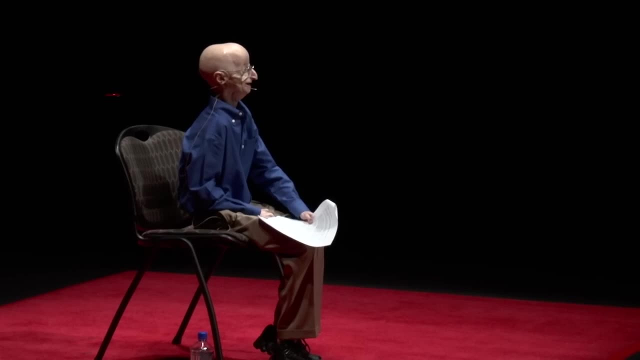 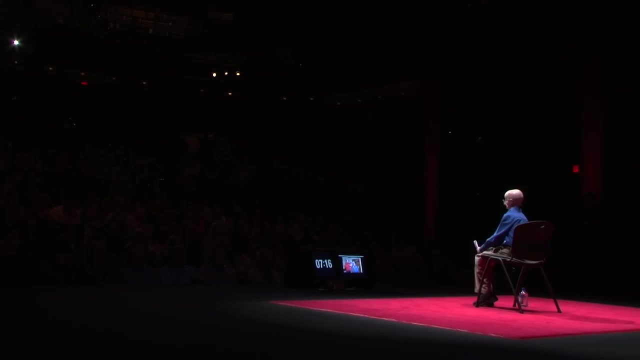 Thank you. So the bottom line here is that I hope that you appreciate and love your family, love your friends for you guys, love your bros and acknowledge your mentors and your community, because they are very real aspects of everyday life that can make a truly significant difference. 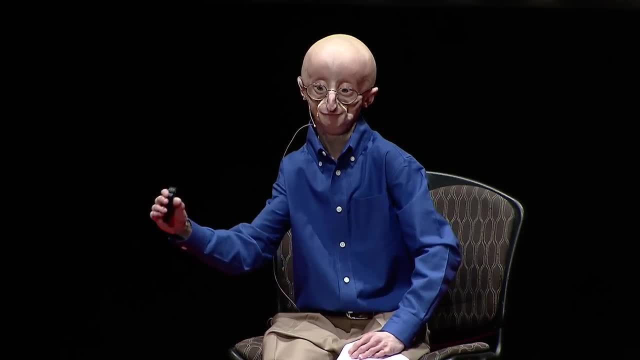 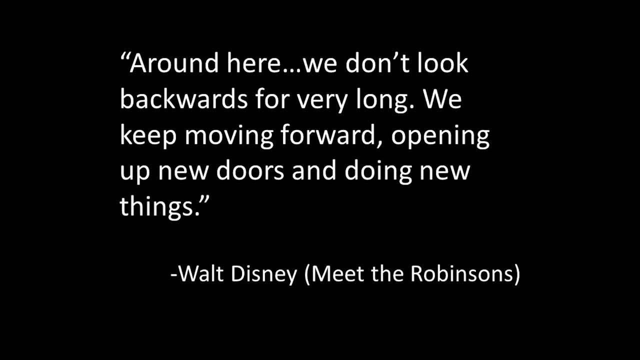 And they can have a positive impact. So the third aspect to the philosophy is keep moving forward. Here's a quote by a man you may know named Walt Disney, and it's one of my favorite quotes. I always try to have something to look forward to. 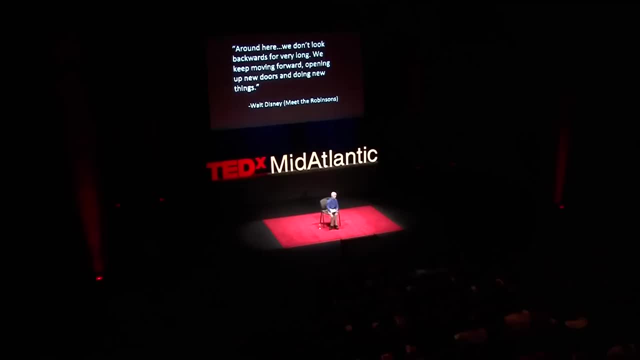 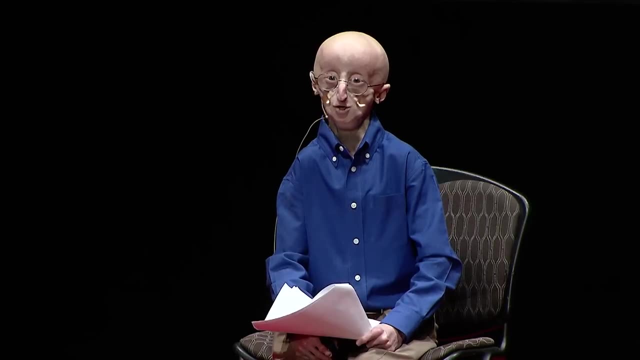 something to strive for to make my life richer. It doesn't have to be big. It could be anything from looking forward to the next comic book to come out, or going on a large family vacation, or hanging out with my friends to go to the next high school football game. 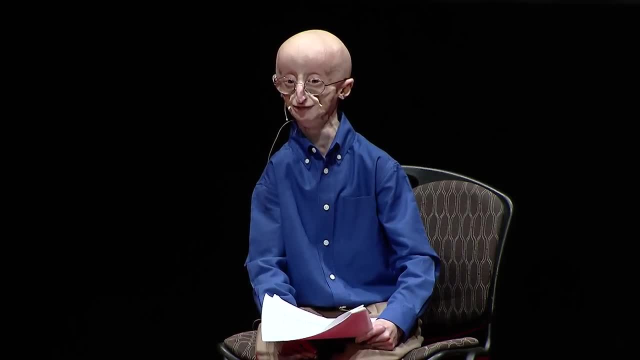 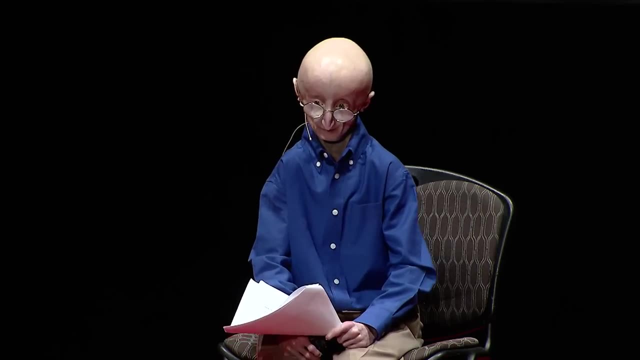 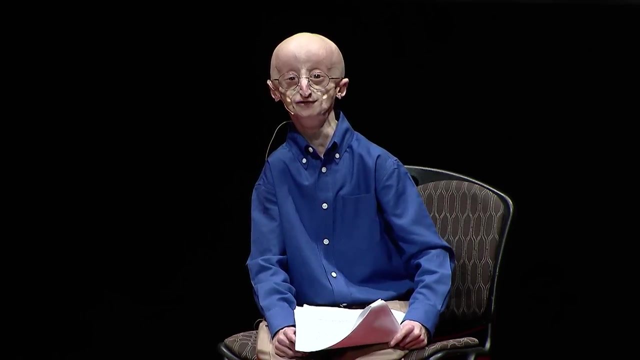 However, all of these things keep me focused and know that there's a bright future ahead and may get me through some difficult times that I may be having Now. this mentality includes staying in a forward-thinking state of mind. I try hard not to waste energy feeling badly for myself. 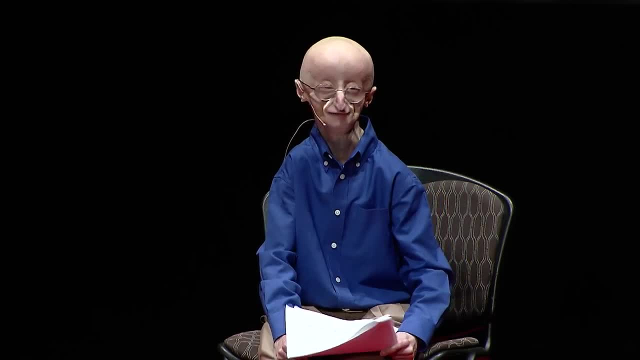 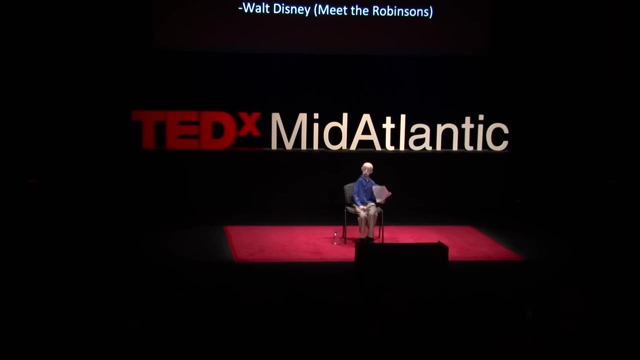 because when I do, I get stuck in a paradox where there's no room for any happiness or any other order, There's no room for emotion. Now, it's not that I ignore when I'm feeling badly, I kind of accept it. 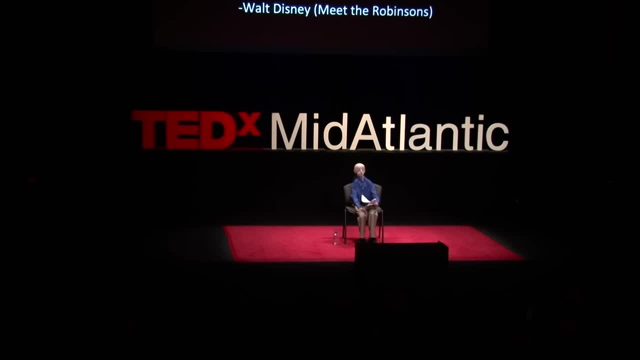 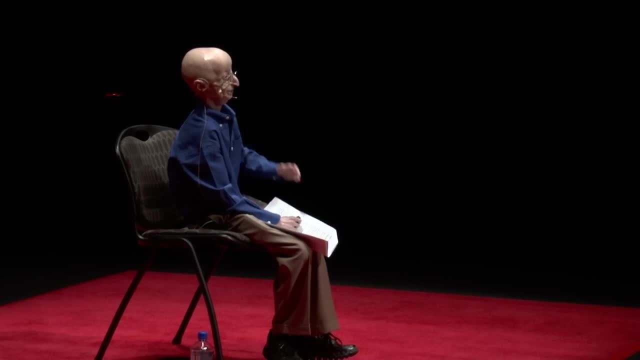 I let it in so that I can acknowledge it and do what I need to do to move past it. When I was younger, I wanted to be an engineer. I wanted to be an inventor who would catapult the world into a better future. Maybe this came from my love of Legos. 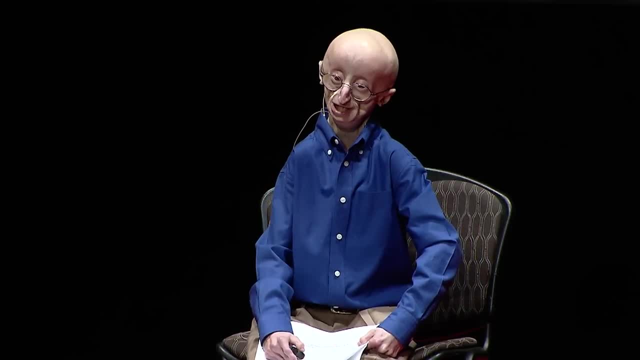 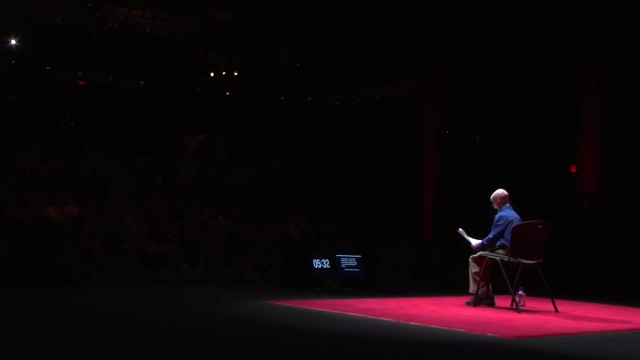 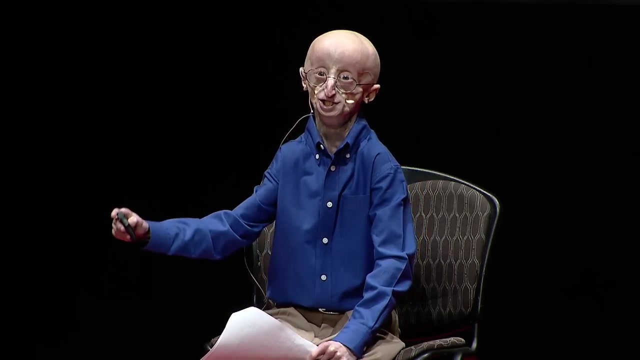 and the freedom of expression that I felt when I was building with them, And this was also derived from my family and my mentors, who always make me feel whole and good about myself. Now, today, my ambitions have changed a little bit. I'd like to go into the field of biology. 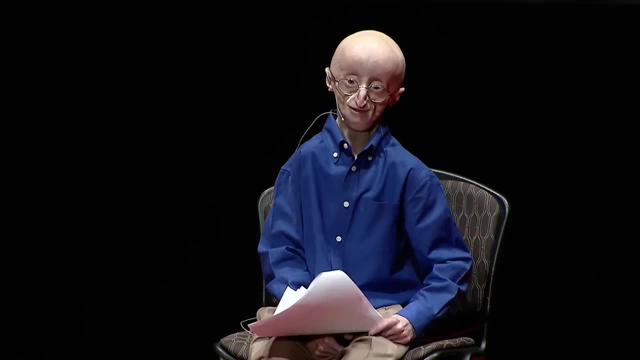 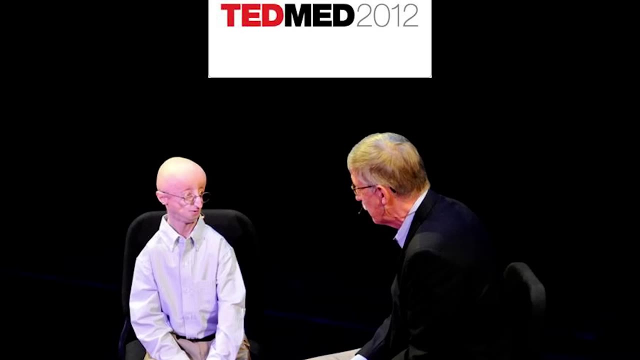 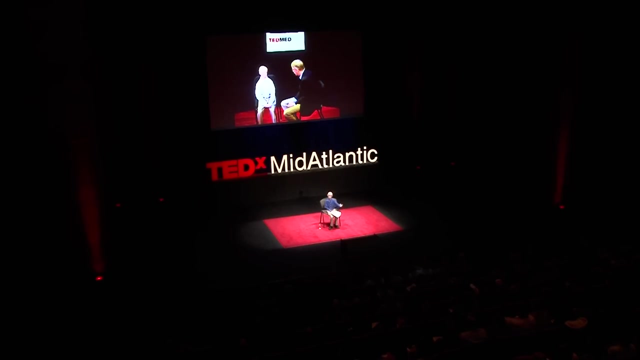 maybe cell biology or genetics or biochemistry or really anything, And this is a friend of mine who I look up to, Francis Collins, the director of the NIH, And this is us at TEDMED last year chatting away. I feel that no matter what I choose to become, 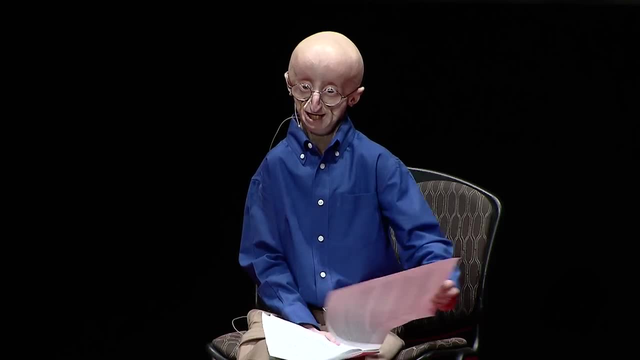 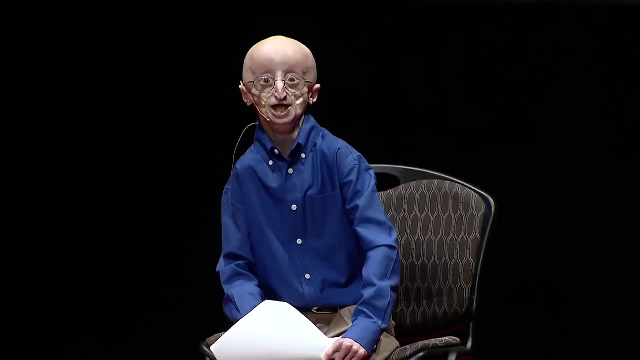 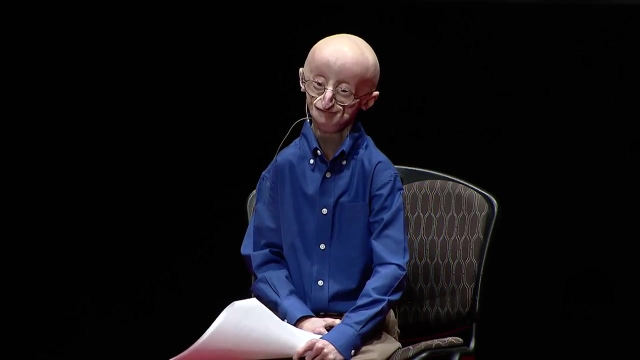 I believe that I can change the world And as I'm striving to change the world, I will be happy. About four years ago, HBO began to film a documentary about my family and me, called Life. According to Sam Now, it was a pretty great experience. 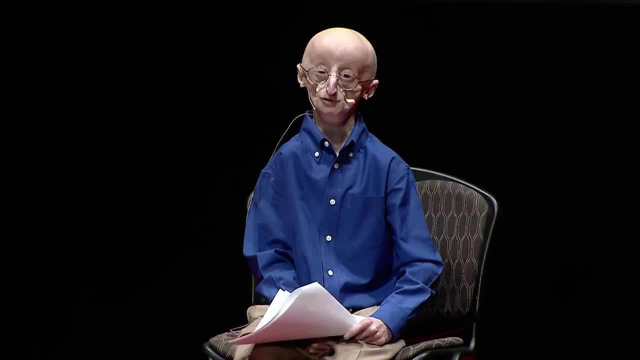 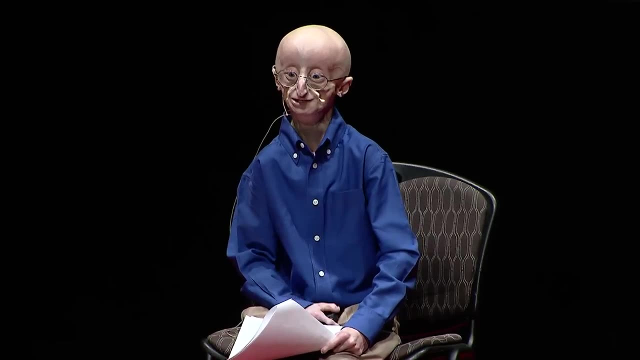 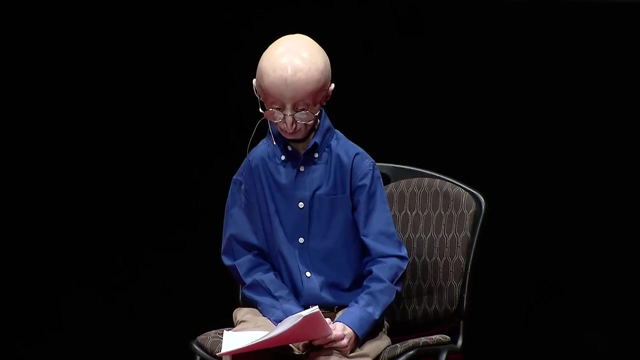 but it was also four years ago And, like anyone, my views on many things have changed and hopefully matured, like my potential career choice. However, some things have stayed the same throughout that time, like my mentality and philosophy towards life, So I would like to show you a clip of my younger self from the film. 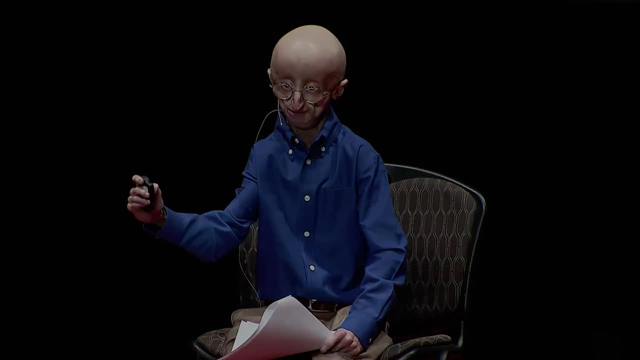 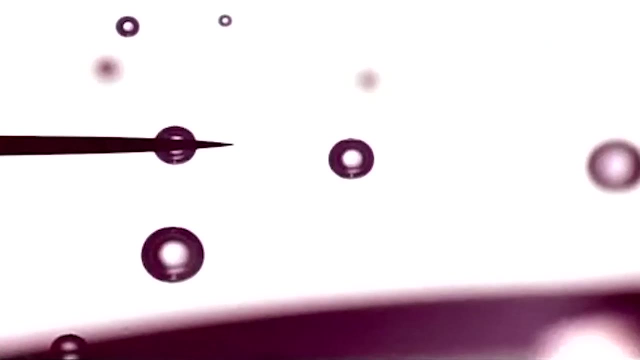 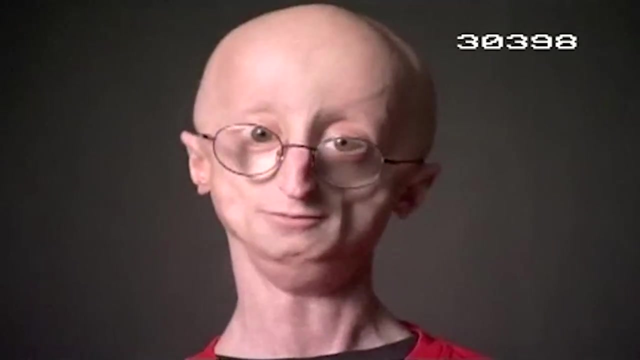 that I feel, embodies that philosophy. I know more about it genetically, So it's less of an embodiment now. It used to be like this thing that prevents me from doing all this stuff, that causes other kids to die, that causes everybody to be stressed. 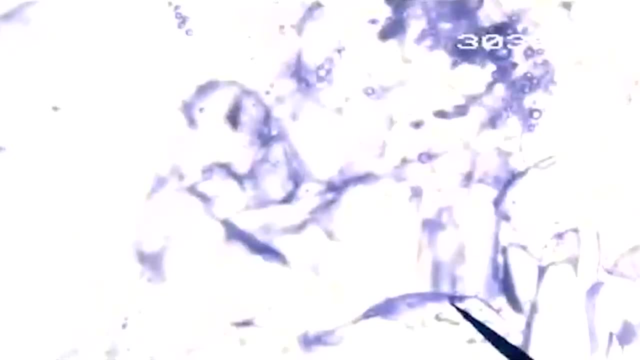 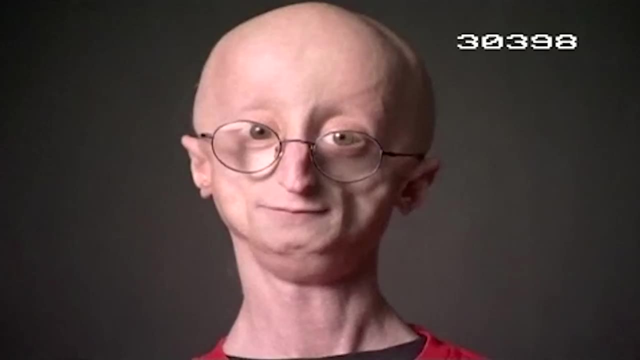 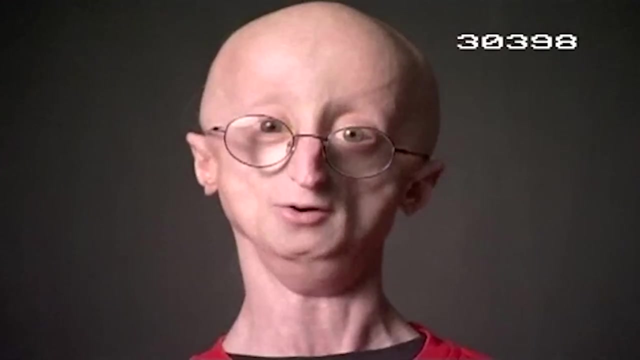 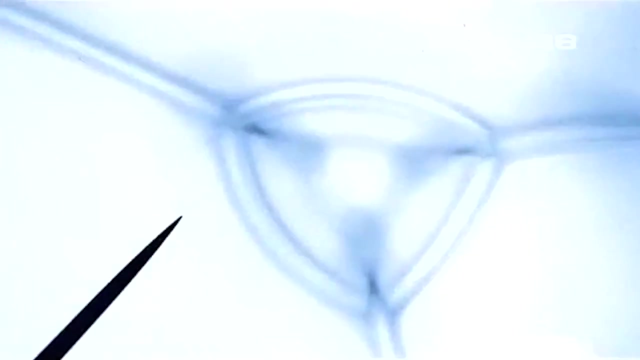 And now it's, you know, a protein that is abnormal, that weakens the structure of cells, And it takes a burden off of me, because now I don't have to think about progeria as an entity. Okay, pretty good, huh? 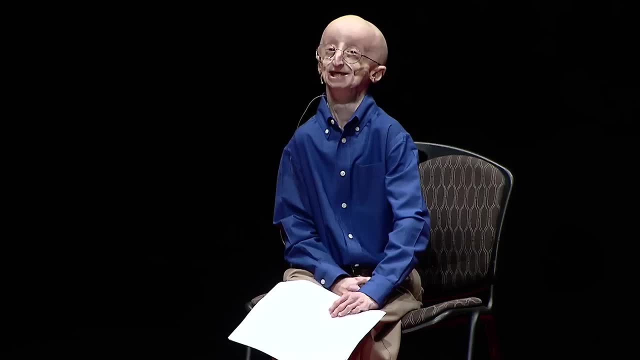 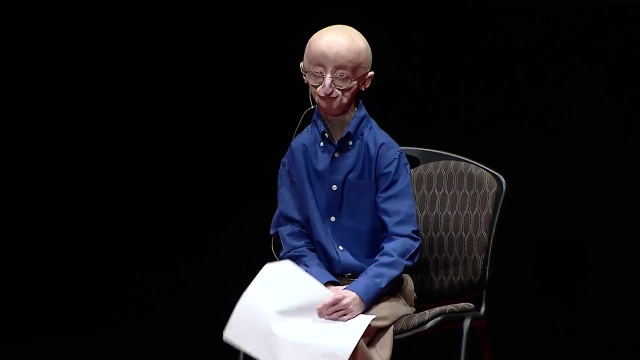 Yep, Thank you. So, as you can see, I've been thinking this way for many years, but I never really had to apply all of these aspects of my philosophy to the test at one time. until last January, I was pretty sick.